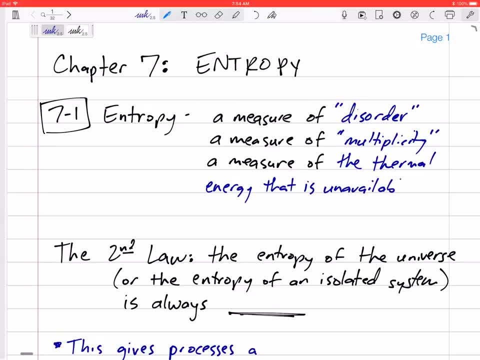 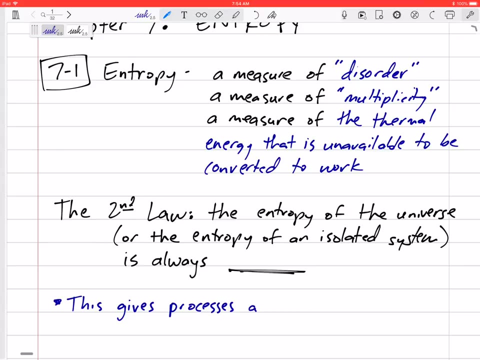 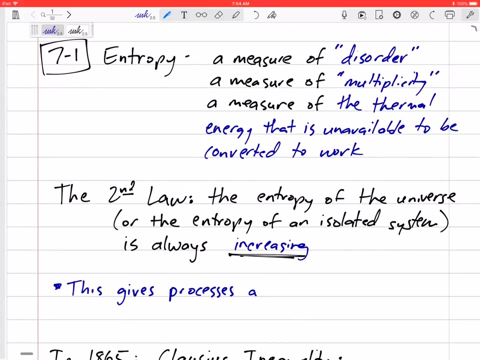 all right, and and we know that the second law of thermodynamics states: the entropy of the universe, um, is always increasing. or. but even if, uh, we're not talking about the universe, the entropy of an isolated system. isolated system is basically: everything is, uh, the you, you know, everything is, um encapsulated into that system. uh, so also the entropy of an isolated 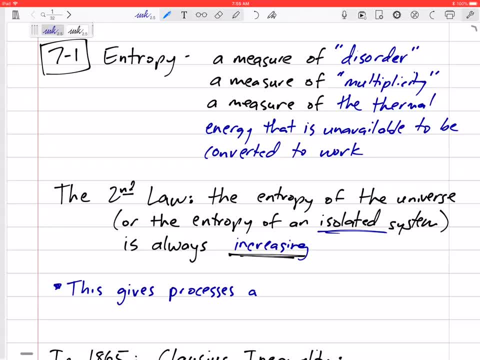 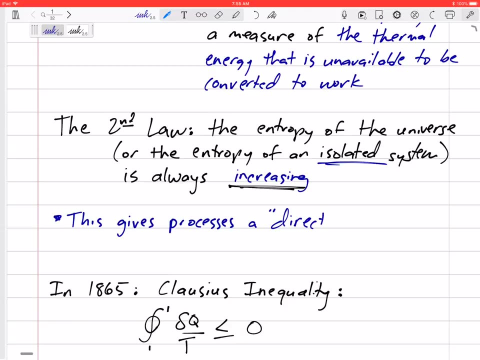 system, a system that you know is isolated, that cannot feel any of its surroundings, any of its boundaries, uh, is also always increasing, all right. so this gives processes a direction because, uh, it must occur in the direction of increasing entropy, must occur in the direction of increasing entropy. 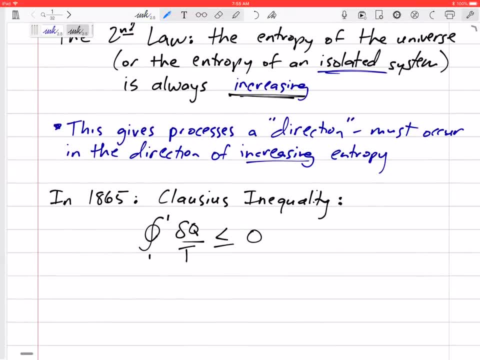 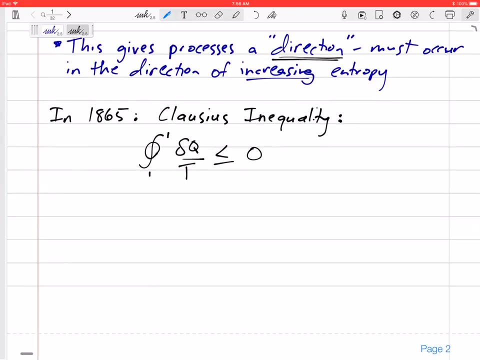 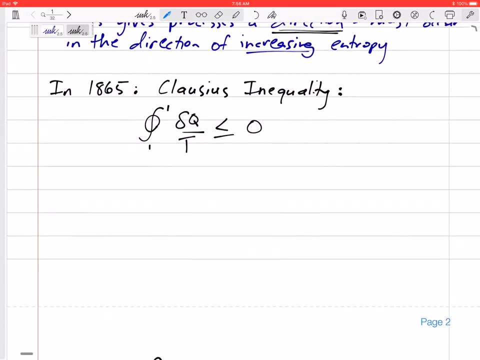 entropy. all right. so we know that um, um processes, you know, have a a certain path, a certain direction, a certain um you know direction that it wants to go and that's in the direction of increasing entropy. all right. so, even way back to uh 1865, uh, clausius uh came up with this, uh, inequality, he, he, he figured out, he um noticed. 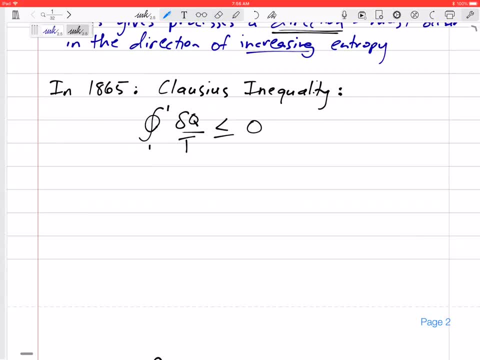 that the integral over a cycle of this value of uh delta q over t- that's just a lowercase delta- it infinitesimally small. differential uh change in q, heat transfer, um. if he integrated that over the whole cycle he found it was always always always negative or zero. it was uh, never positive. 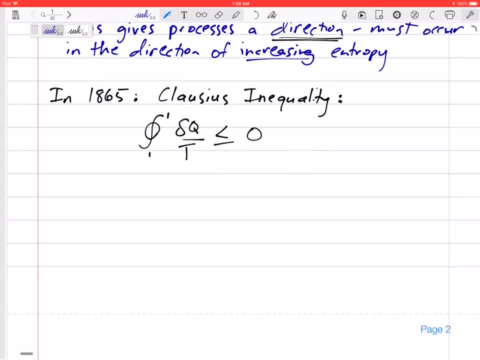 all right. so let's let's write this um integral in words. now, this, uh, this thing, right here, it's just an integral. so this is integration over the whole cycle. right, if something's going from from one and then eventually it comes back to state one, if you. 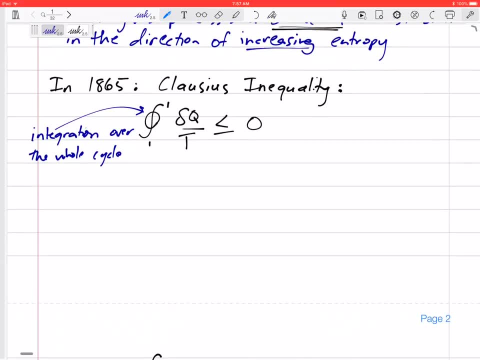 integrate it over the whole process. it's a cyclic um integral. so let's write this um, let's write this equation in words. it's the cyclic integration or the cyclic integral of delta q divided by temperature is always less than or equal to zero. the sum of all 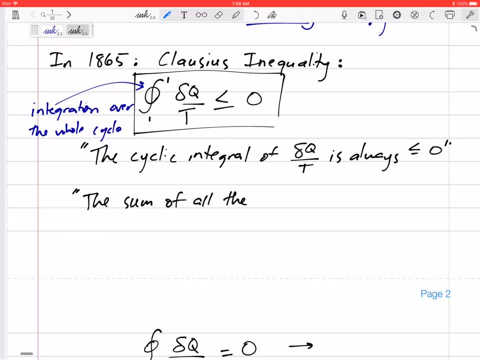 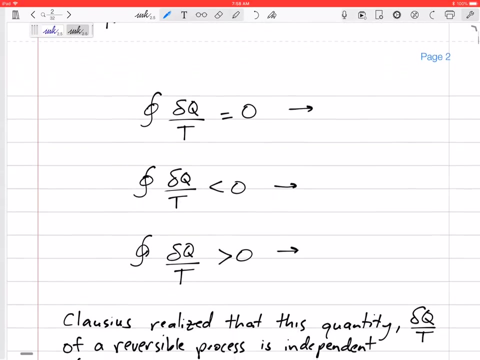 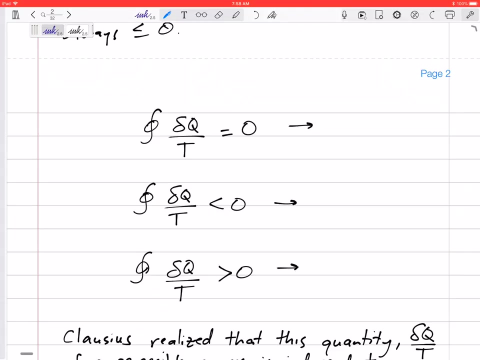 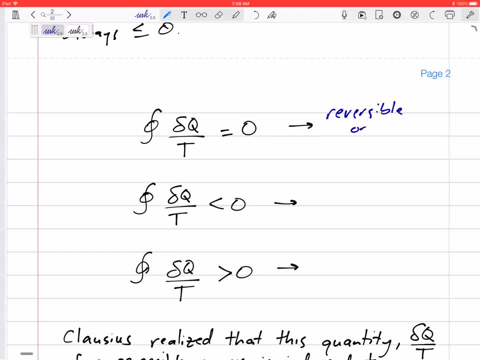 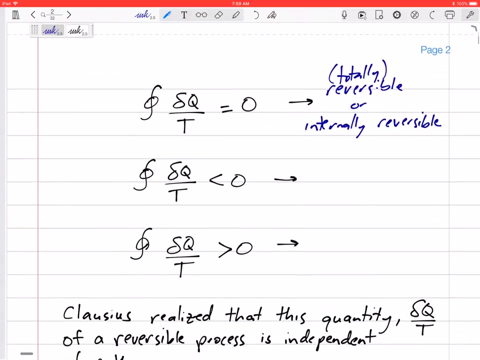 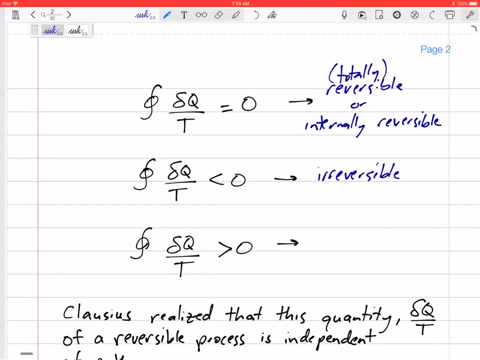 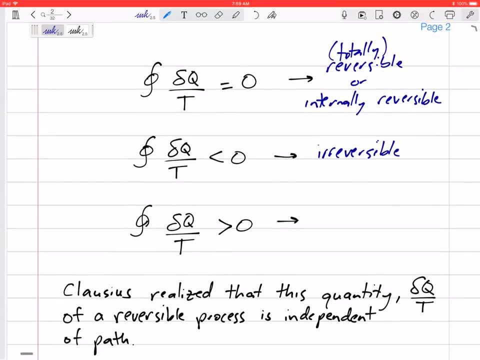 a most of our processes are is negative. but the cyclic integral delta q over t, the cyclic integral delta q over t, this never happens. this is impossible. it's never positive. so at at clausius realized: was that this quantity of heat that you're going tonatally? 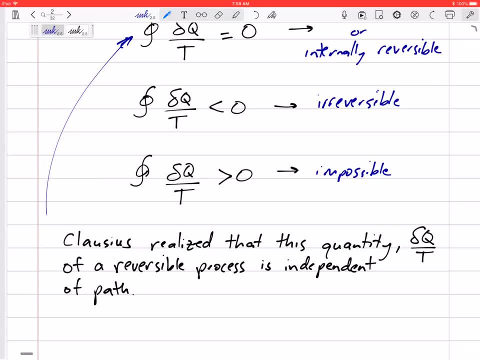 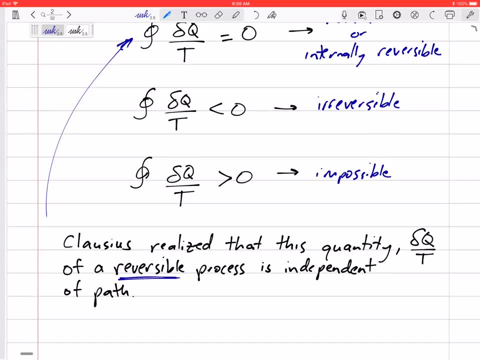 study of delta Q over T of a reversible process, it came back to zero. no matter what, no matter what, what path it went on, whether it went from 1 to 2, to 3 to 4, to 5, to 6, back to 1, or just from 1 to 2 and back to 1, as long as it came back to 1. 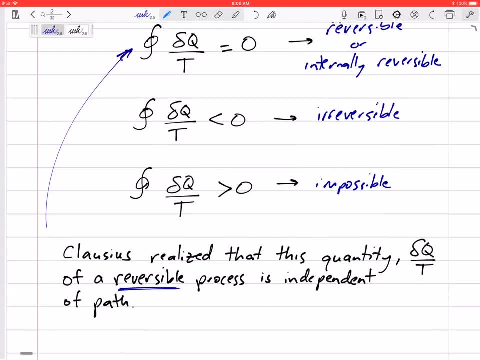 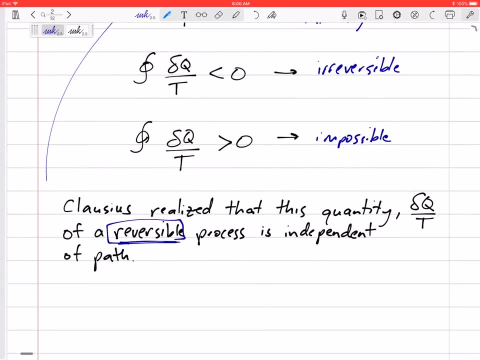 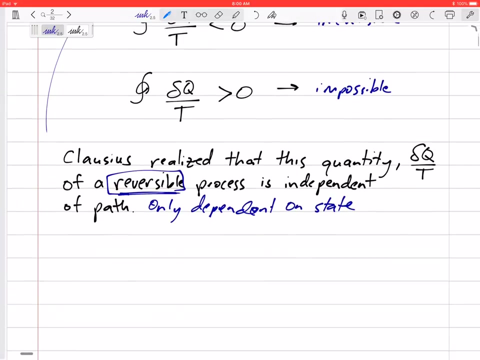 it was equal to 0, and so it was. it didn't change. it was independent of the path, of a reversible process, right? it was only dependent on the state, and so he realized that this is a new state variable. so let's say he discovered a new. 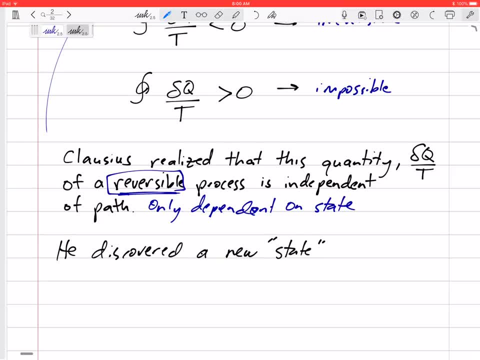 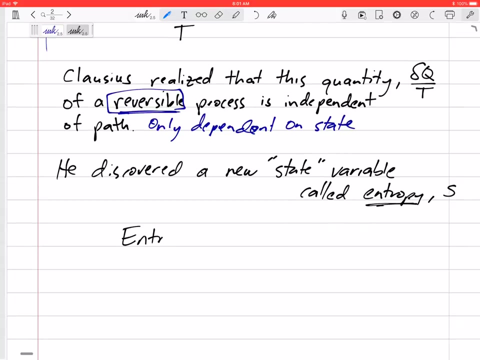 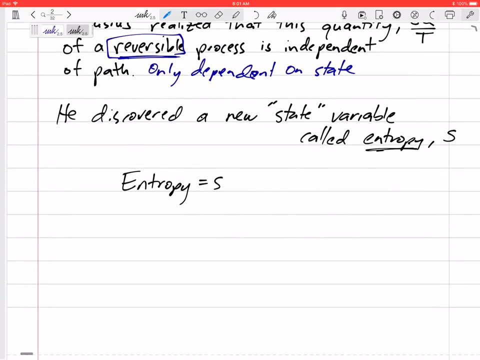 variable, state variable variable that is independent of the path, and we're going to call this entropy. we're going to call this entropy now and we're going to call entropy s. so let's say entropy. a measure of disorder is defined as s, and 여러분PRINTSCH modified s in a different form, and so we're actually. 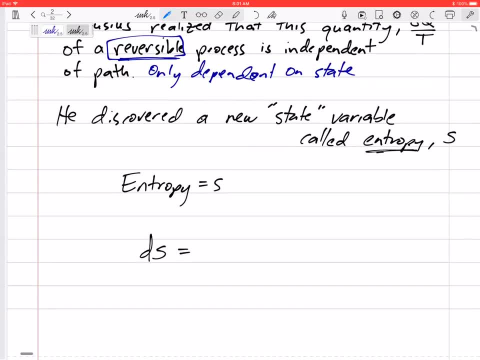 to define this as ds, a differential and infinitesimally small change in S is pin of Ac Metropolitan S التي MIRROR 0 for an internally reversible or total reversal process. all right, so ds is equal to dq over T of an internally reversible process. 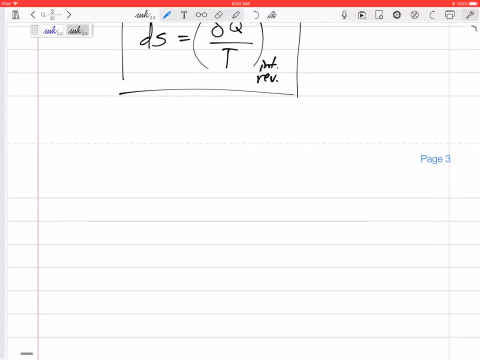 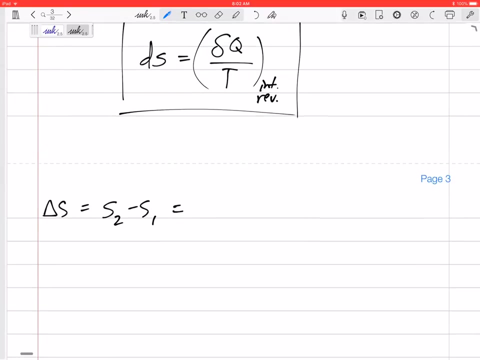 So if we took the integral of both sides then we would have S2 minus S1.. So the change in entropy S2 minus S1, and we need to take the integral of that. delta Q over T is equal to the integral of delta Q over T from 1 to 2. 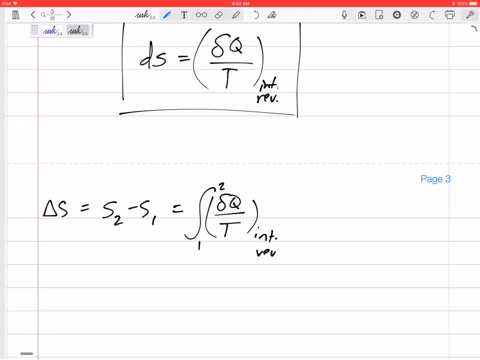 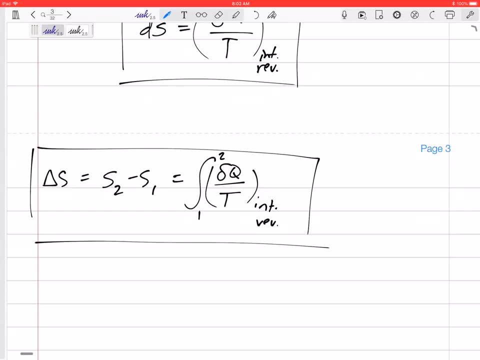 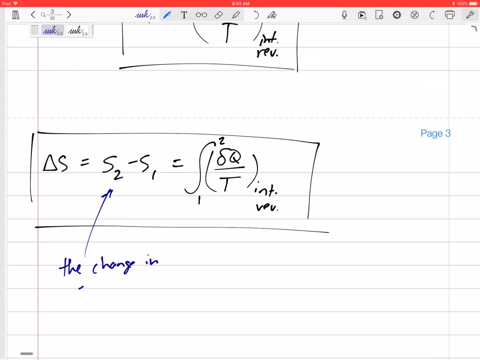 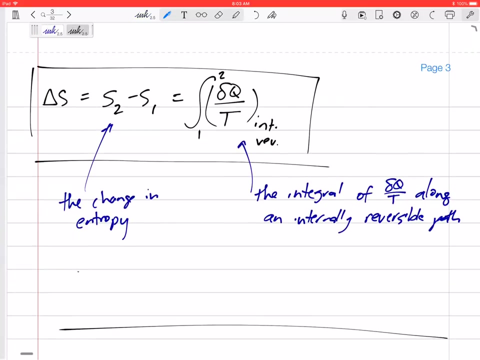 of an internally reversible process. So let's box this in and let's write this in words: The change in entropy. the change in entropy is defined as the integral of delta Q over T along an internally reversible path. Okay, Now these two could be capital S total entropy. 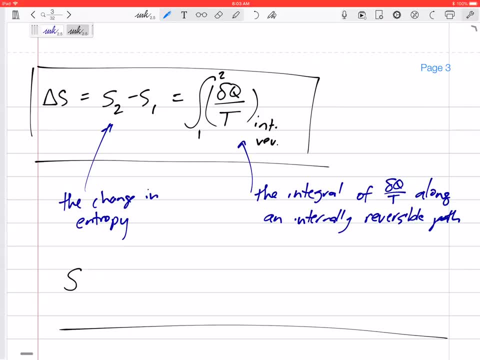 or lowercase s specific entropy, So capital S, we'll just call it. entropy would be in kilojoules per K. You notice that this is per temperature And lowercase s specific entropy has units of kilojoules per kilogram K. 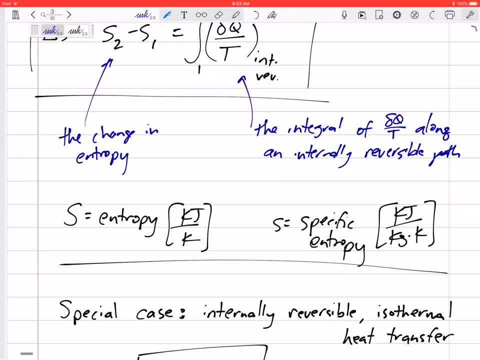 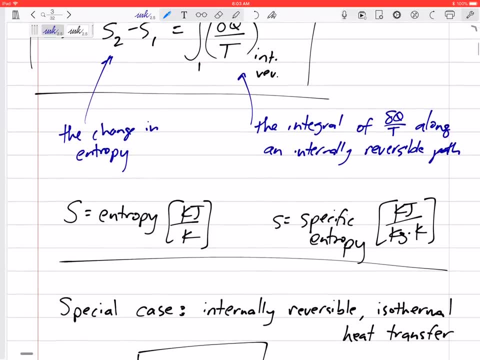 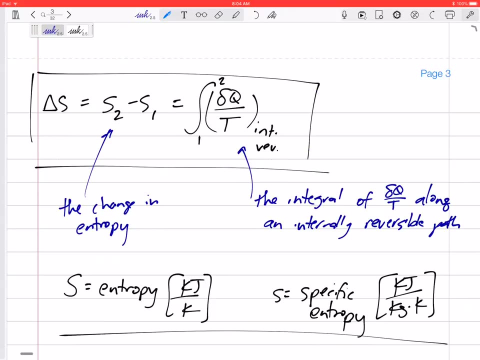 So it's a little bit different than some of our other properties because because of this it's per temperature, per Kelvin, Okay, But that's, that's pretty tough, right? You know? this is the change. is is equal to an integral of delta Q over T. 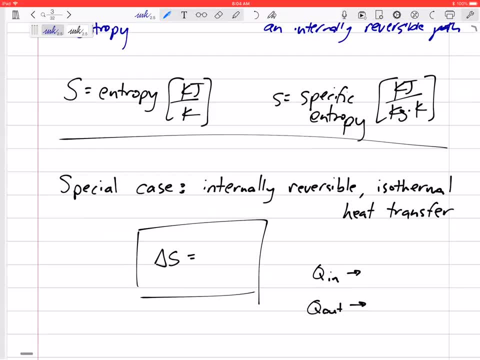 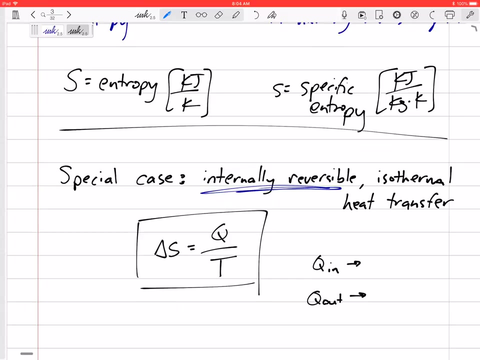 But we're lucky that there are some special cases. All right, So for an internally reversible isothermal, right. So temperature: temperature is constant, heat transfer: Delta Q is just Q over T. All right, So we can find the change in entropy of a process of a. 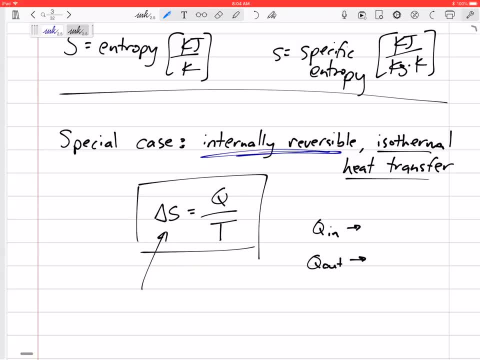 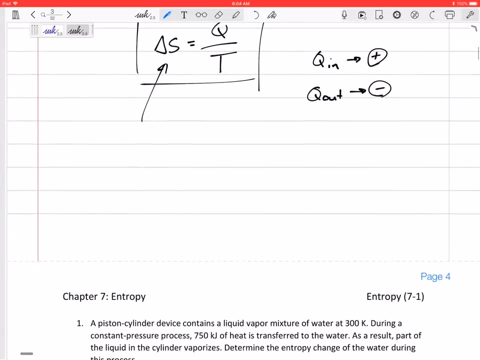 an isothermal heat transfer process is just equal to Q over T. Q in is positive Q, Q out is negative Q. Now we have to get the heat transfer. that's negative Q. All right, So let's do an example real quick.